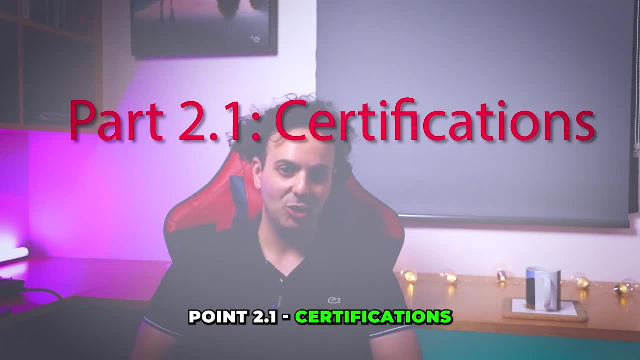 courses in the description box below Point 2.1.. Certifications: It's not about the piece of paper, it's about the knowledge that you gain. If you're just starting out, then this is a video where I go through certifications. 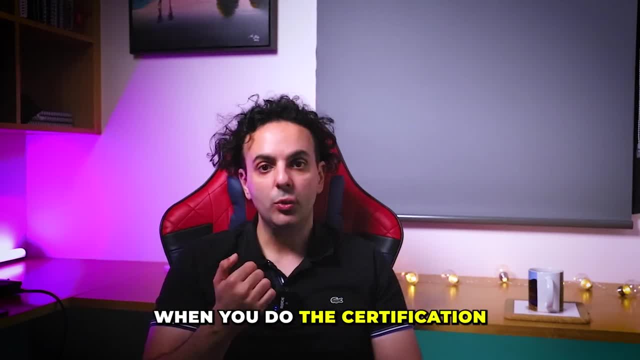 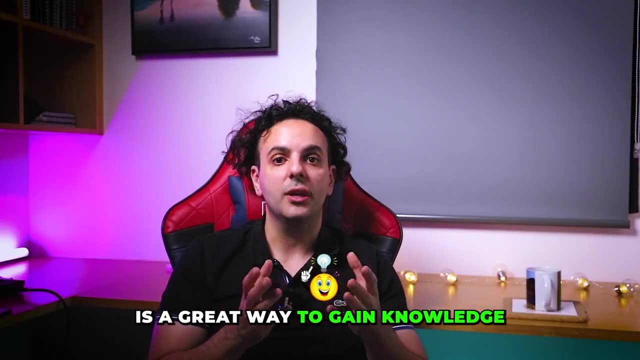 but I recommend to someone who is completely new to cyber security: When you do the certification, you see the process of studying for an exam and passing that exam in its itself is a great way to gain knowledge into a certain topic. In my opinion, the best way of learning cyber. 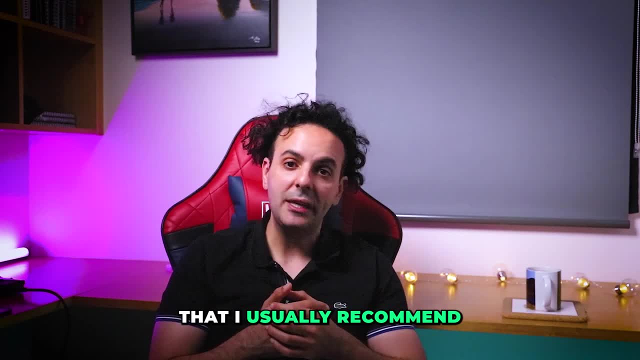 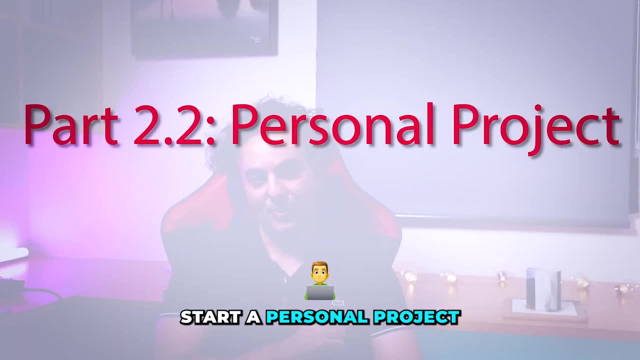 security is by doing, and those certifications that I usually recommend are practical and hands-on, meaning you need to pass a lab exam in order to get the certification. Point 2.2.. Start a personal project As you're doing the certifications I want you to pick. 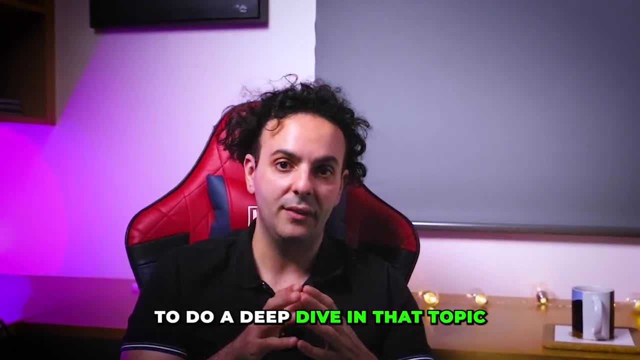 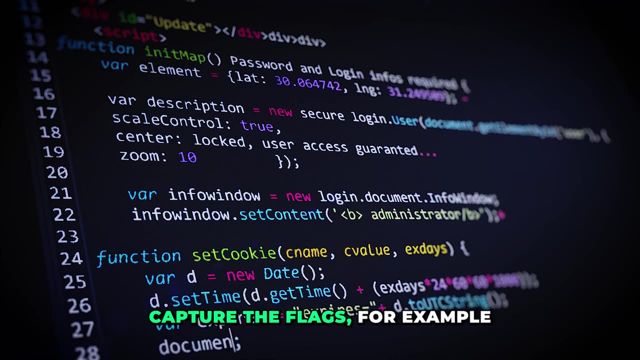 a topic that you're mostly interested in, Like, for example, this one. But if you're just it in and I want you to do a deep dive in that topic- For example, if you decide that you want to become a penetration tester- then I want you to start a personal project where you do capture. 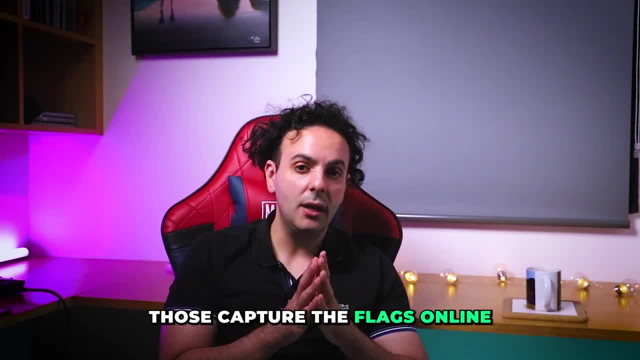 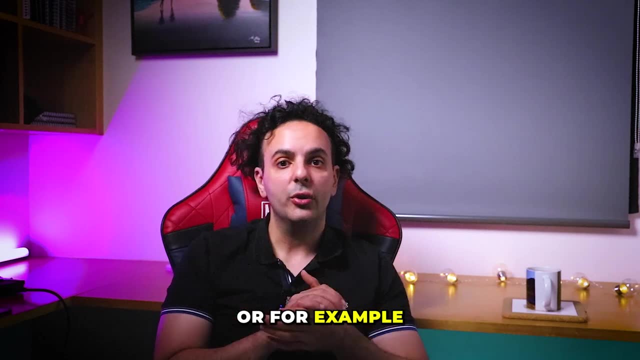 the flags, for example, and you can find those. capture the flags online, or you can do them through something like hack the box or try hack me, or even in events that you will find in your community. Or, for example, if you decide to be a blue team professional or a security operation. 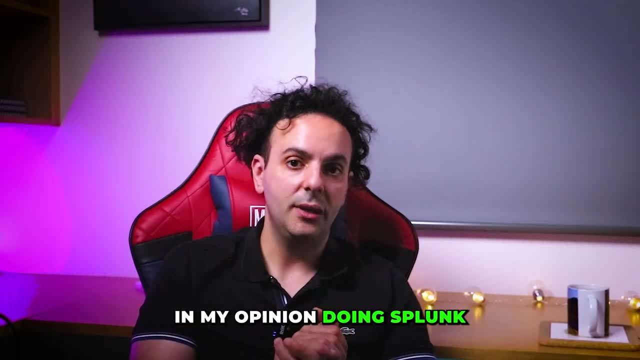 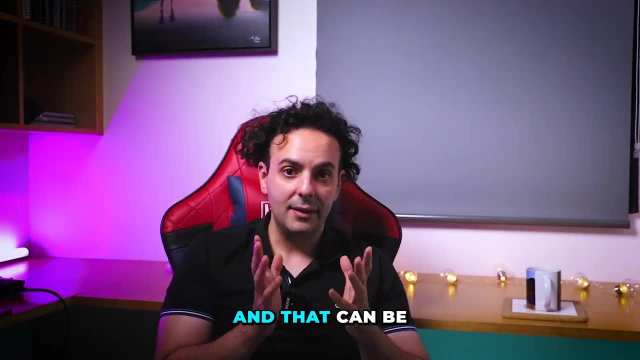 analyst in a SOC, then pick a tool and get really good at it. In my opinion, doing Splunk training and certifications, which are completely free, is an excellent way for someone who wants to become a SOC analyst And that can be your personal project. You can do things with Splunk. you can. 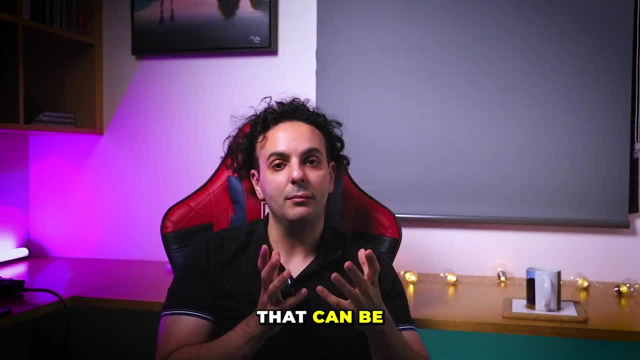 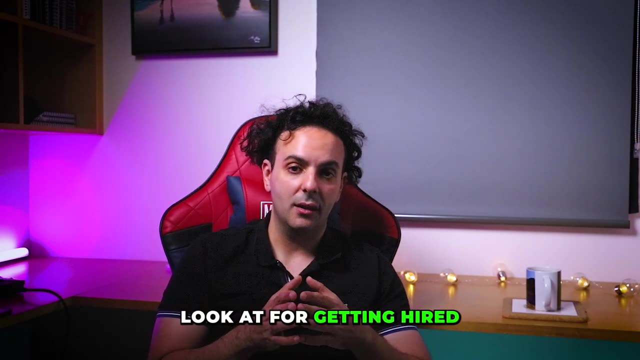 search, you can do queries, you can write your own little scripts in Splunk. That can be your personal project which you can put into your CV. Which brings me to the last point: getting hired. The first thing that you need to look at for getting hired is your CV. You can be the best cyber. 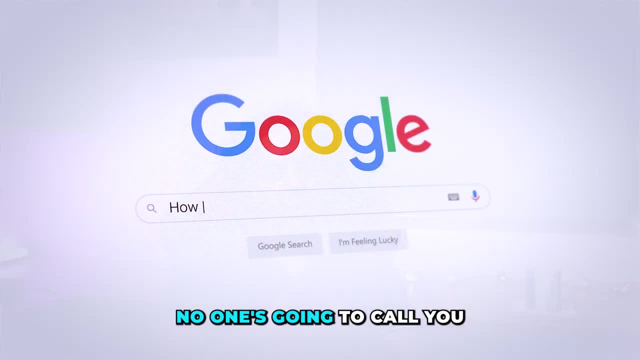 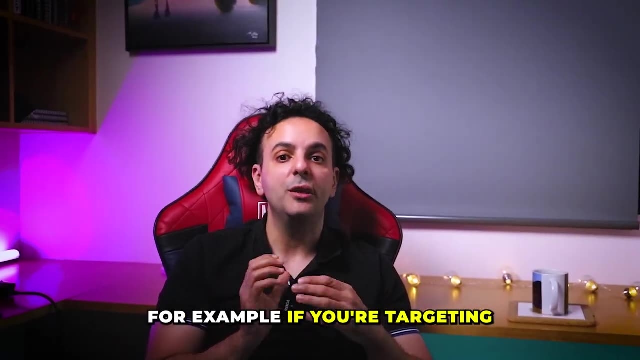 security professional in the world. but if your CV is bad, no one's going to call you for an interview. And the most important part of your CV is the practical skills and the tool and the knowledge that you have. For example, if you're targeting penetration testing, 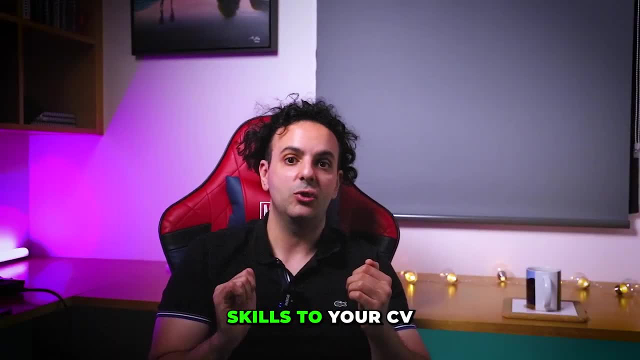 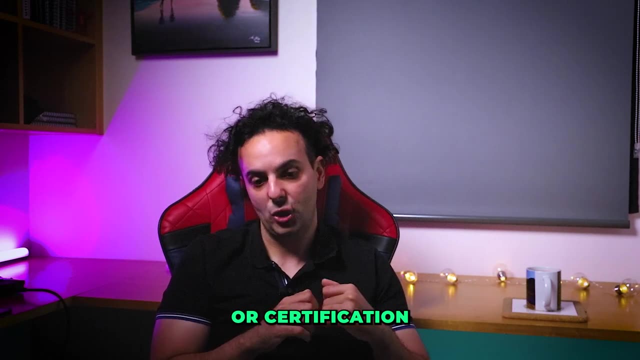 job. it's really, really important to add specific skills to your CV, So talk about your experience using particular tools that you use in your penetration, testing, personal project or certification. The same thing applies if you're looking for a SOC analyst role as a beginner. 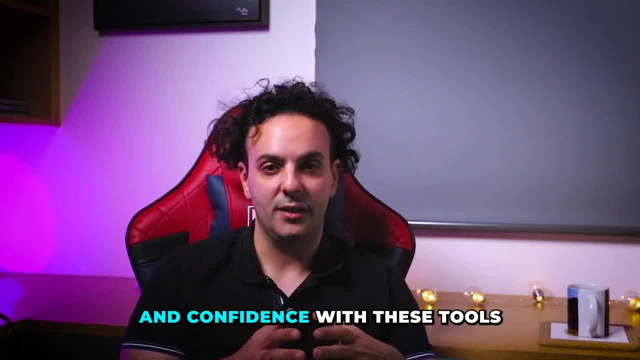 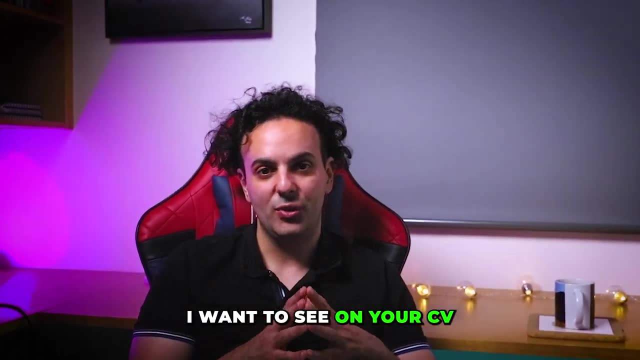 is to add the tools that you've learned and got some experience and confidence with these tools. For example, if you've been doing Splunk certifications and you have a personal project doing Splunk work, then the first thing I want to see on your CV is that work you've 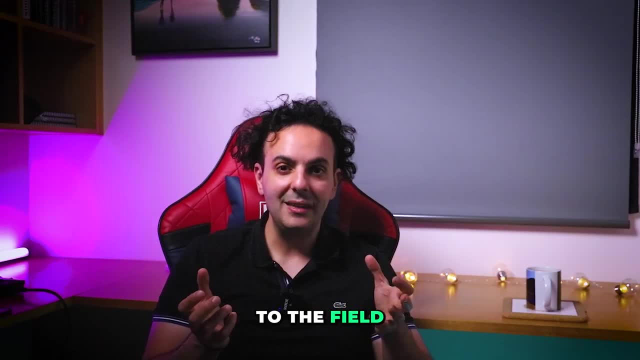 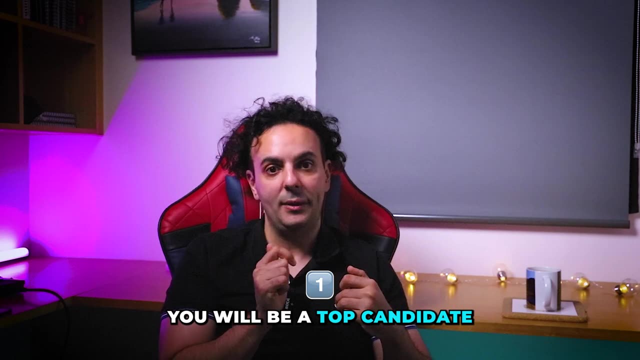 done with Splunk. As a hiring manager, we know that someone who's new to the field doesn't have all the knowledge that we need. But if someone who's a beginner show me that they know a specific tool that we used in the job, trust me, you will be a top candidate And 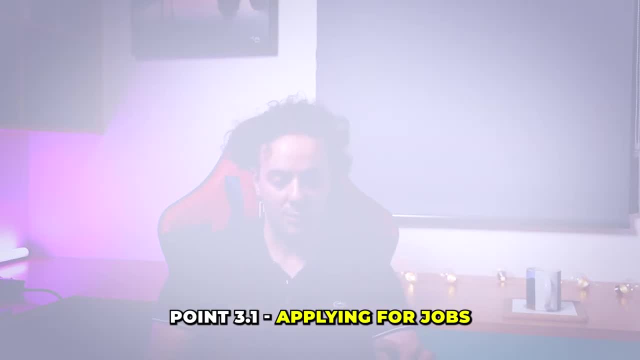 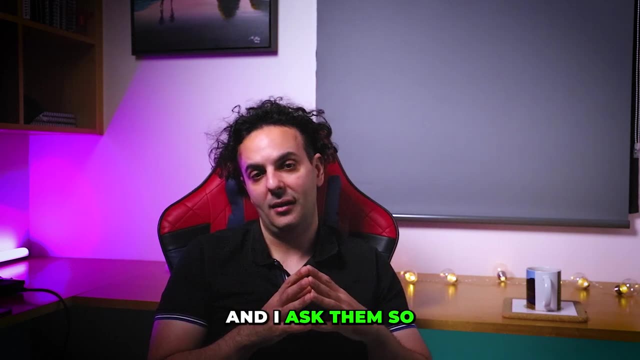 I want to interview you. Point 3.1, applying for jobs. This one drives me crazy, especially with people that I mentor. I usually get someone who is trying to break into cyber security and I ask them: so how many jobs have you applied to? And they'll: 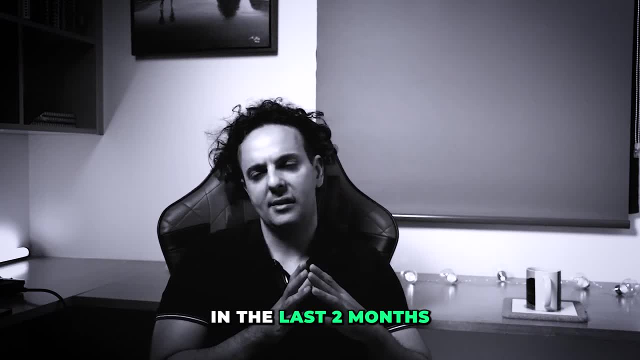 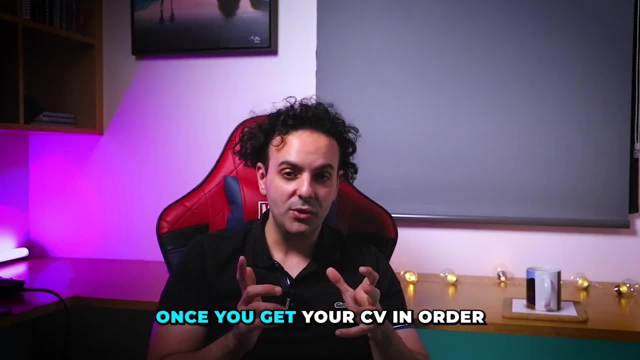 be like I applied to maybe one or two jobs in the last two months and I got rejected. You can't do this As a beginner. you can't afford not to apply for jobs Once you get your CV in order. I want you to apply to every single job that you see. I want you to look. 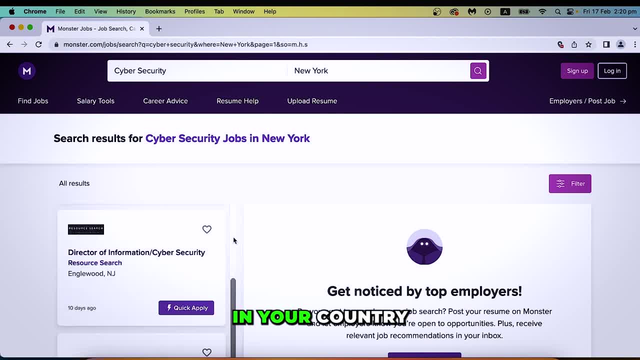 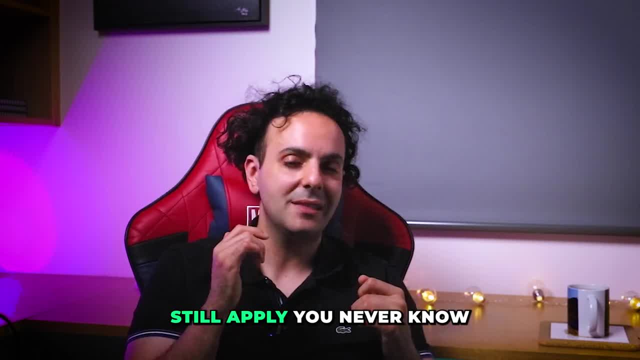 at all the jobs that are advertised on LinkedIn or any job search website in your country every single day, And I want you to hit that apply button. Even if you meet 10% of what they want in that particular job still apply. You never know. As a beginner, you need to. 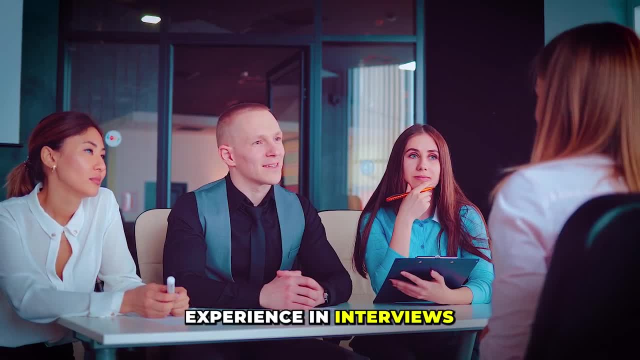 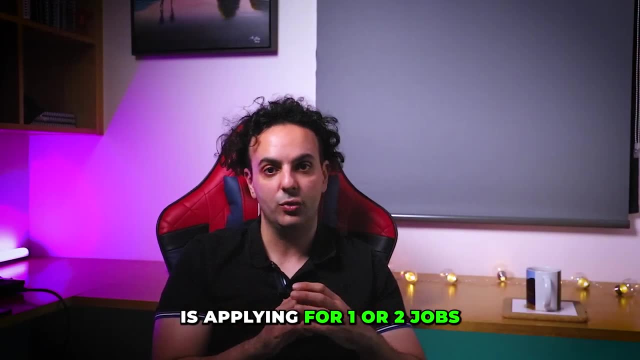 get in front of companies as many times as possible. You need to gain experience in interviews. You need to gain that confidence in talking about your skills In interviews, and this cannot happen if all you're doing is applying for one or two jobs. Point 3.3, the interview. Remember the mindset that we talked about in the beginning. 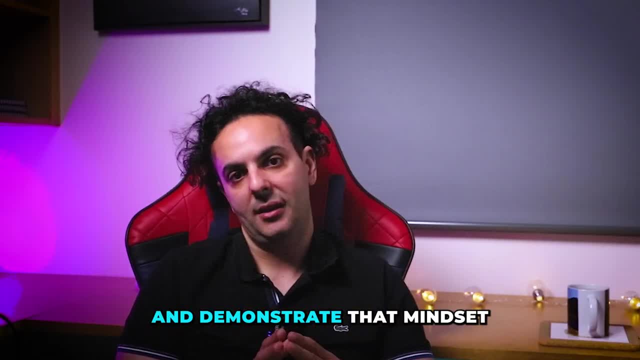 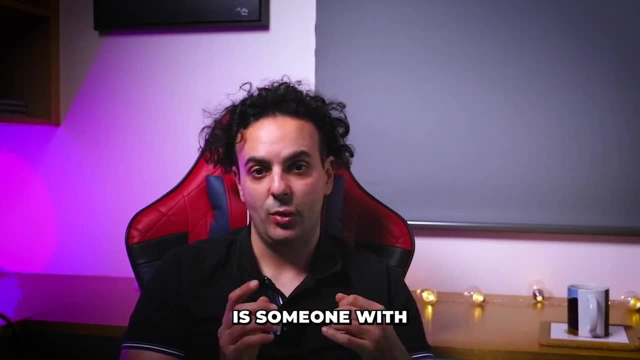 of this video. Now, this is where I want you to display and demonstrate that mindset. When we're hiring for entry level jobs, we know that they don't have all the skills that we're looking for, But what we're really looking for is someone with a good attitude, someone 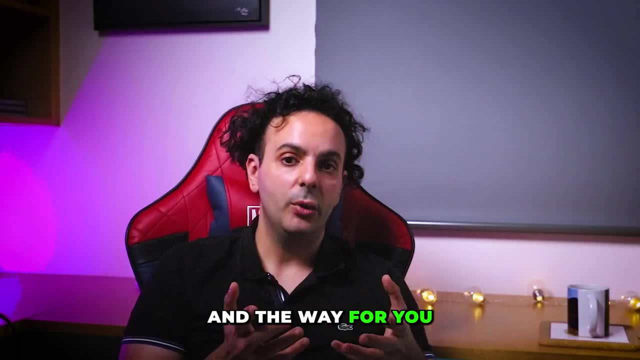 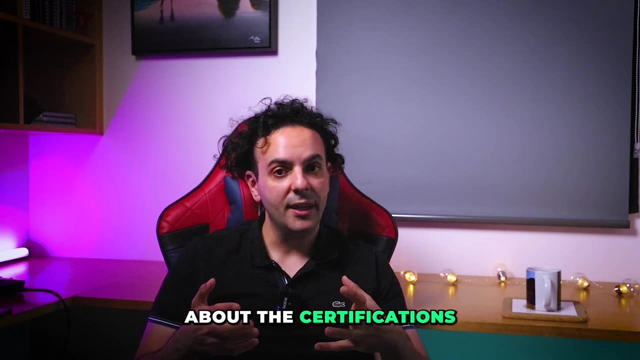 who's willing to learn and someone who can work well with others, And the way for you to demonstrate that is to let us know about the personal project that you've been working on. If you're an interviewer about the certifications that you've been doing, in fact, I want you. 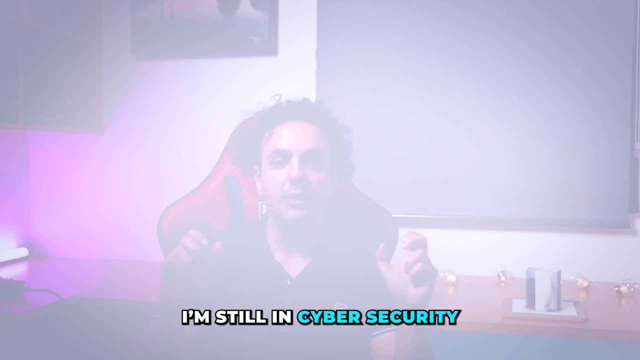 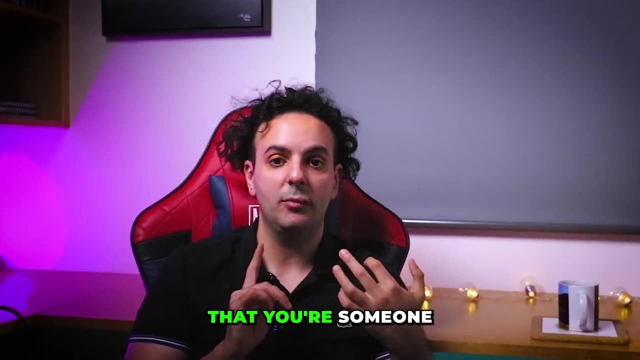 to say this in the interview. I know that I'm still new in cybersecurity, but I'm willing to learn. If there is something that I don't know, I will figure it out and I will learn it. This communicates that you're someone with good attitude, that you're someone with 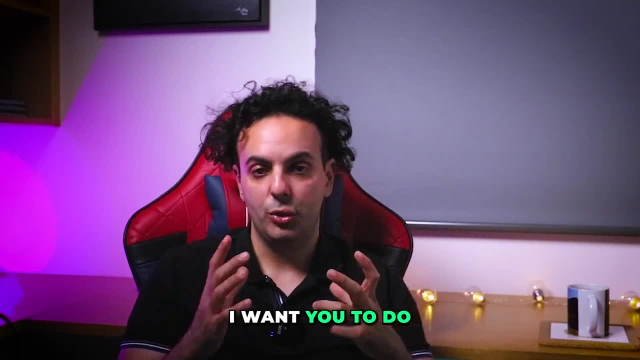 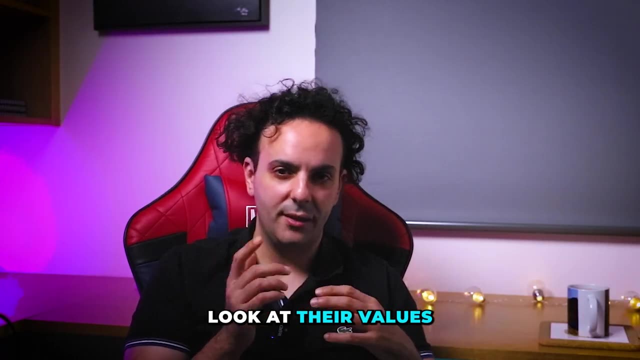 an open mind or not arrogant, and you're willing to learn. The other thing I want you to do before an interview is to actually search the company. For example, if you're interviewing with an insurance company, just have a look at their website, look at their values, look at what is it that they do, Bonus points for those.